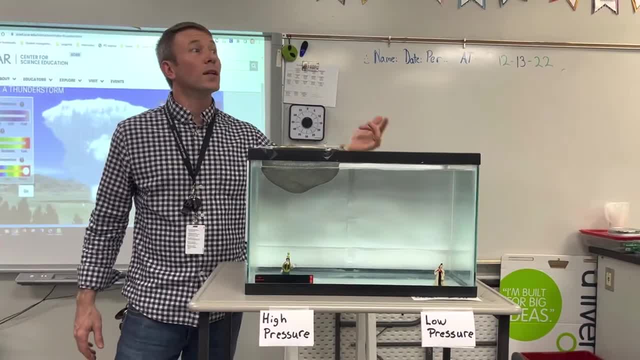 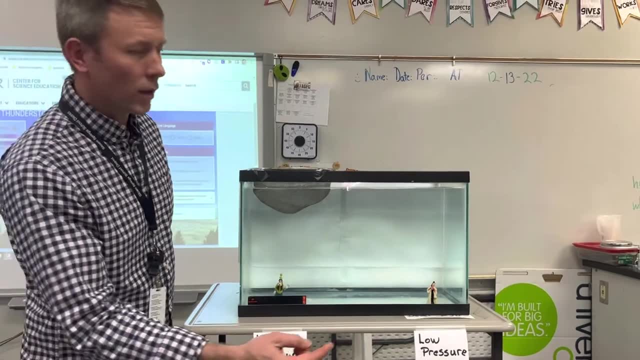 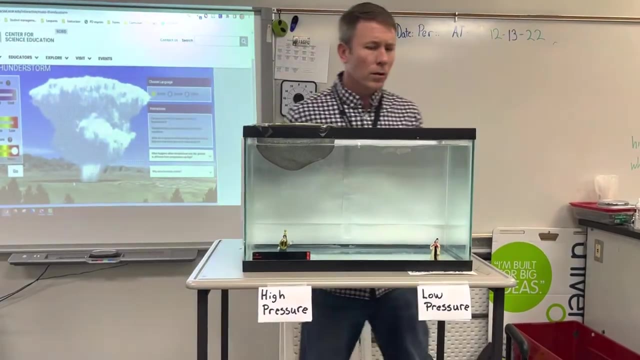 So the question now is what kind of conditions would create a high-pressure area And what kind of conditions in the atmosphere would create a low-pressure area. Well, let me show you what I'm going to do to create the high- and low-pressure systems. 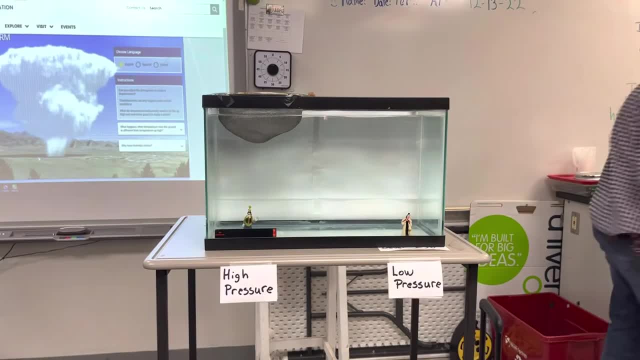 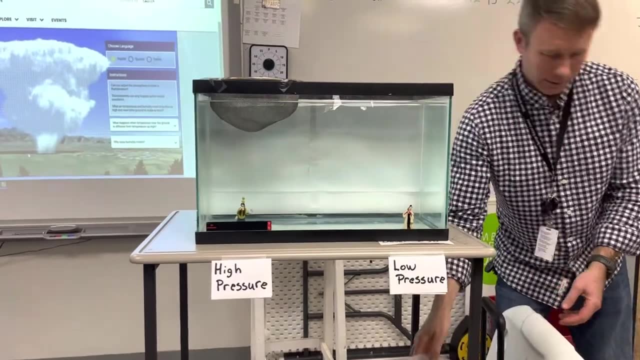 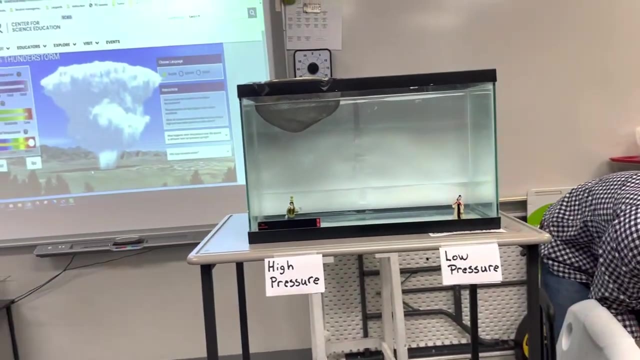 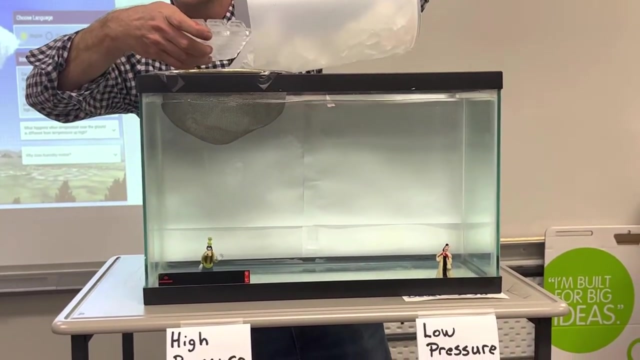 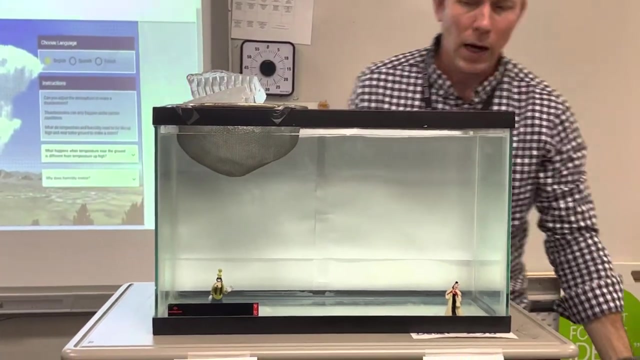 First of all, over on this side where the high-pressure system is going to develop. I'm going to add some ice. I'm going to put that ice right up here in my little strainer, which keeps it all in one spot, keeps it on this side of our system, our model. 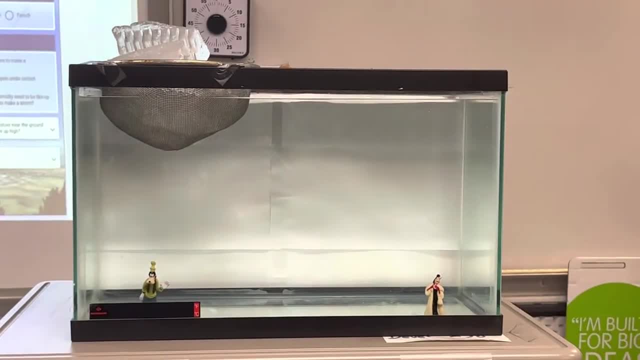 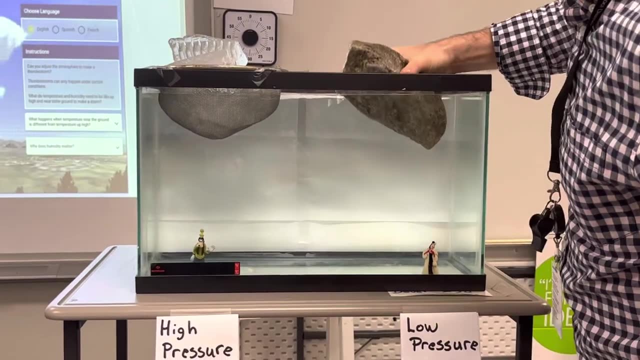 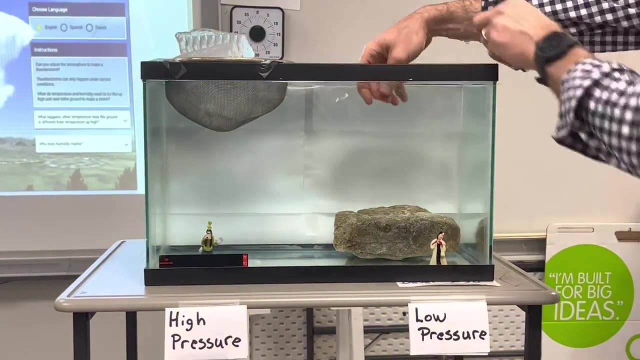 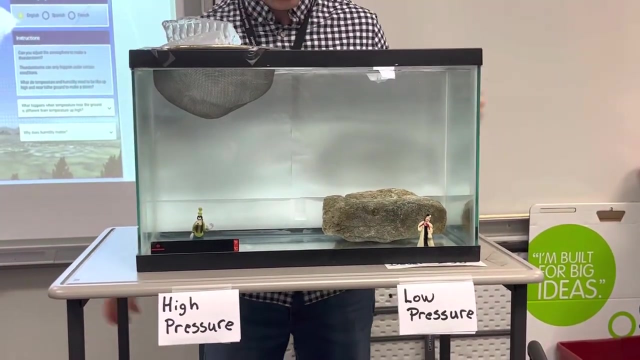 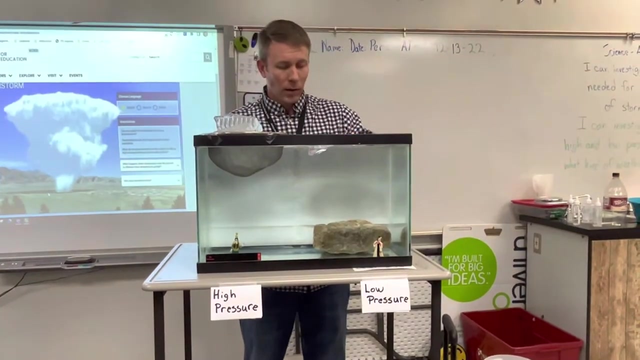 On the other side I'm going to put a rock that I've been soaking in really hot water, So this would be like the ground. okay, It's like the ground that's been warmed by the sun. Now, if we look now, we really don't see anything. but the beautiful thing about using water to represent our atmosphere is: I can go ahead and put some food coloring in it and we can see the movement in our model atmosphere. 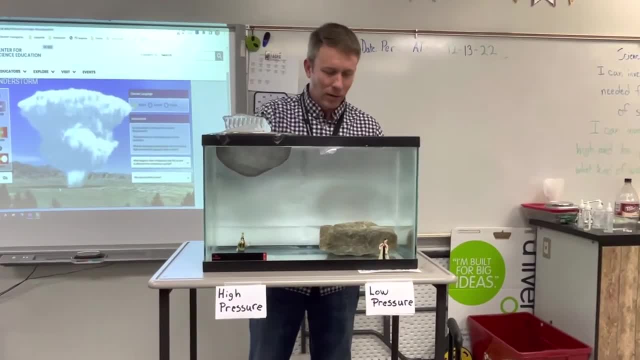 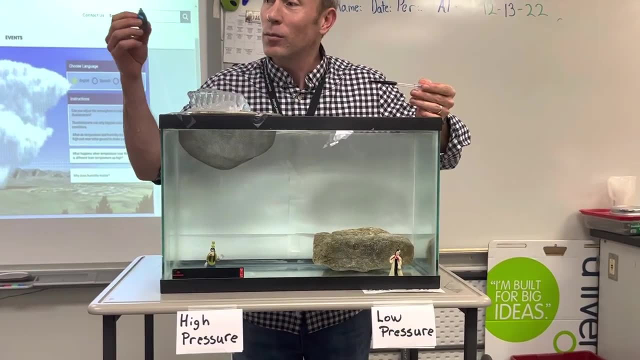 So what I'm going to do here is I'm going to inject some red food coloring on our warm earth and I'm going to put some blue food coloring on our warm earth, and I'm going to put some blue food coloring on our warm earth. 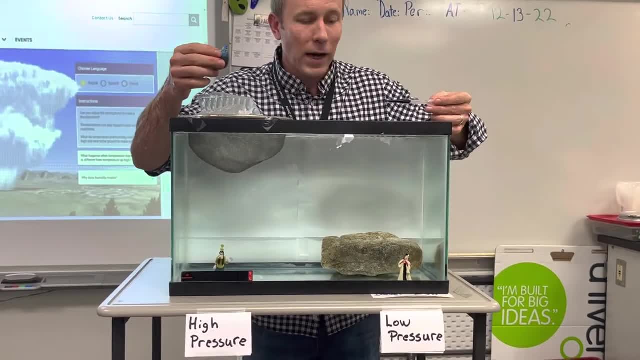 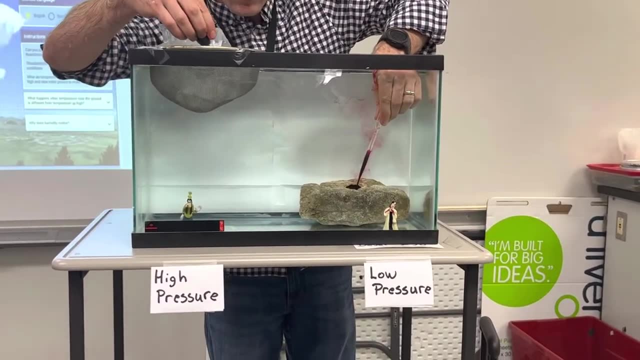 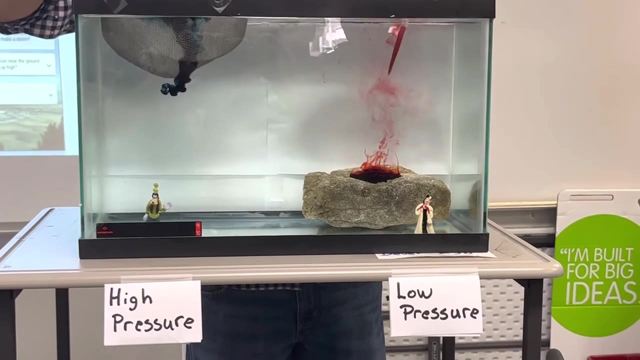 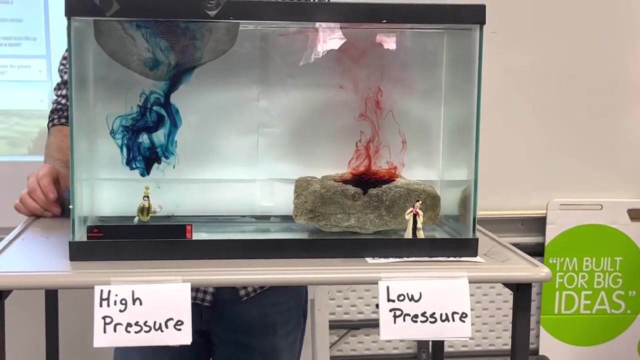 and I'm going to put some blue food coloring in our cold upper atmosphere and let's watch what happens. Okay, let's just wait a minute. I'll be real quiet and watch what occurs here in our atmosphere. Okay, let's just wait a minute, I'll be real quiet and watch what occurs here in our atmosphere. 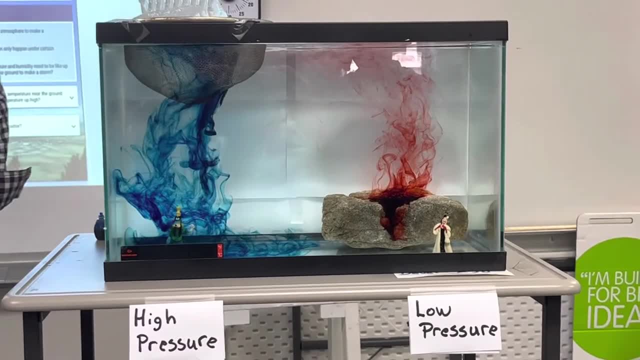 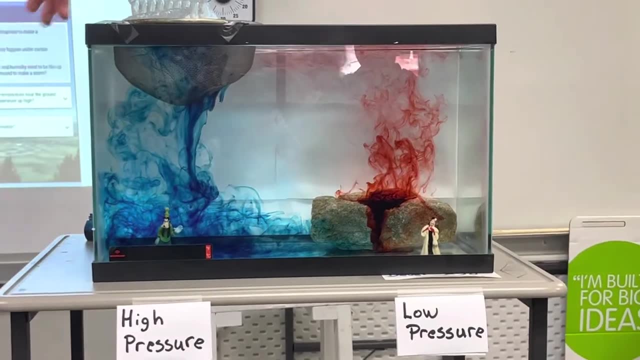 Okay, let's just wait a minute. I'll be real quiet and watch what occurs here in our atmosphere. If we look over here, we can see that the atmosphere over here is cold and dense and falling. It's pushing down on Goofy. That's high pressure when something's pushing down on you.